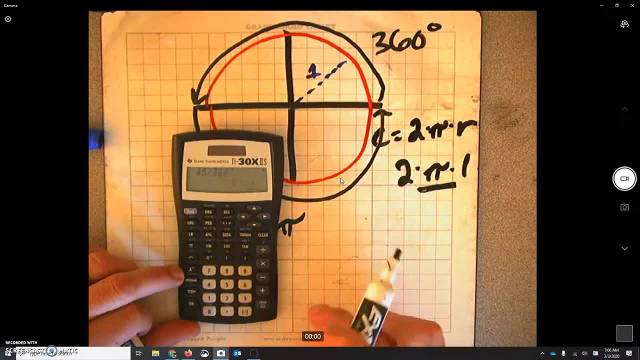 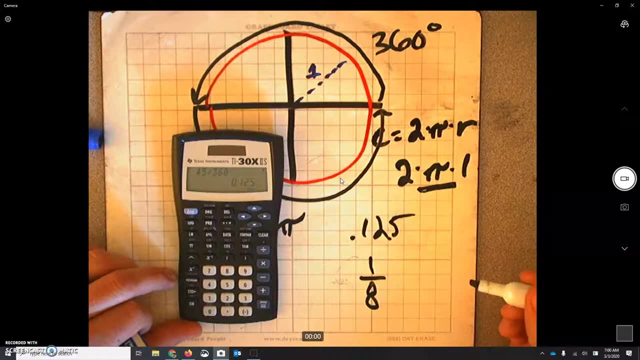 So we have- or I should do it the other way- 45 divided by 360.. We have 0.125, or it's 1 eighth of a circle. So we can do 2, 1 pi times 2 pi, which gives us 2 pi over 8.. 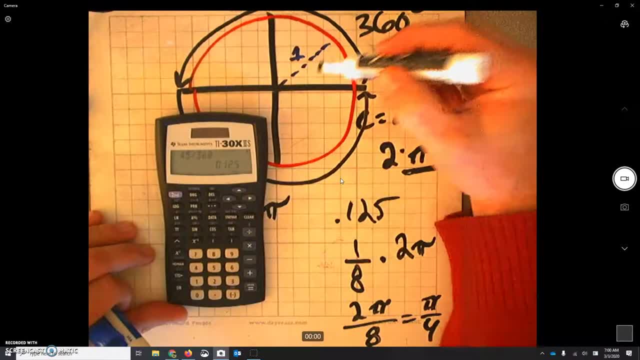 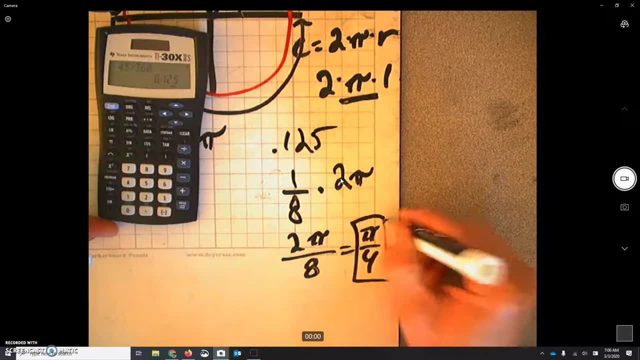 Or just 1 pi over 4.. So a 45 degree angle in a right- sorry- in a unit circle can also be referenced as pi over 4.. All right, we're going to go over this more in detail later. 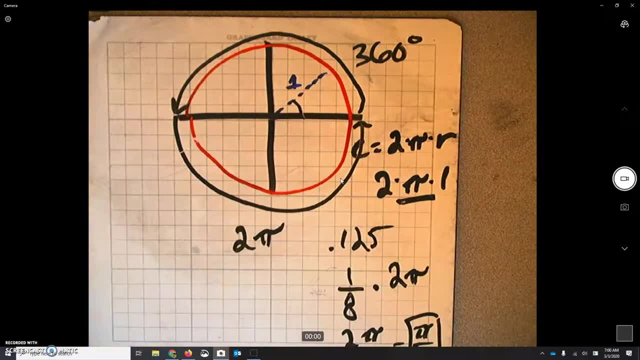 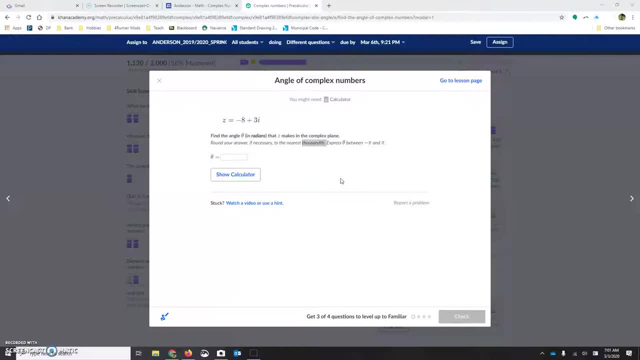 I just want to know, I just want to point out what a radians is while we are answering these questions. Okay, so now let's go back to our question. The point was 8, negative 8 plus 3i. Okay, so let's first plot negative 8 and plus 3i. 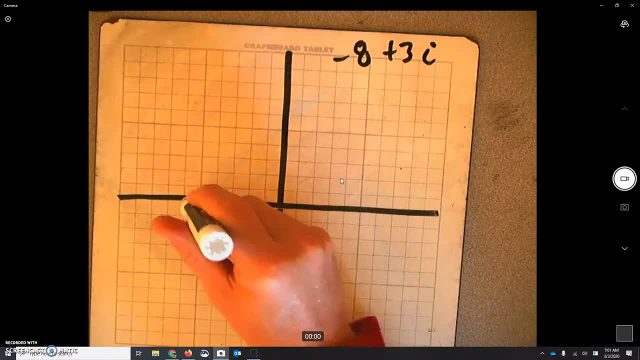 All right. so negative 8 goes 1,, 2,, 3,, 4,, 5,, 6,, 7,, 8.. And negative or positive 3 goes 1,, 2, 3.. So we're going to go right here. 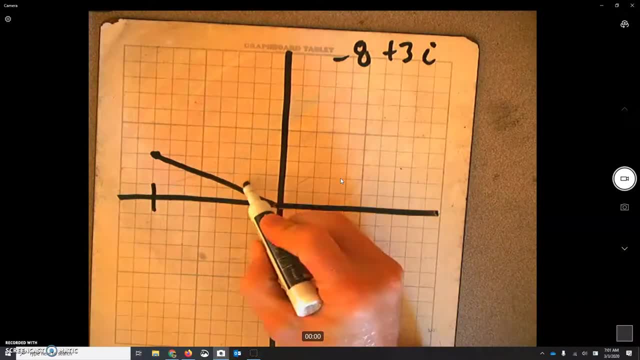 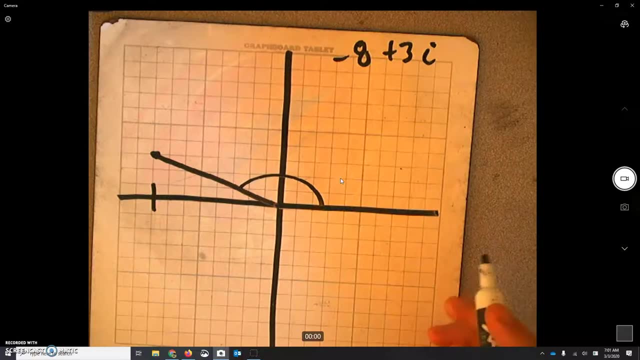 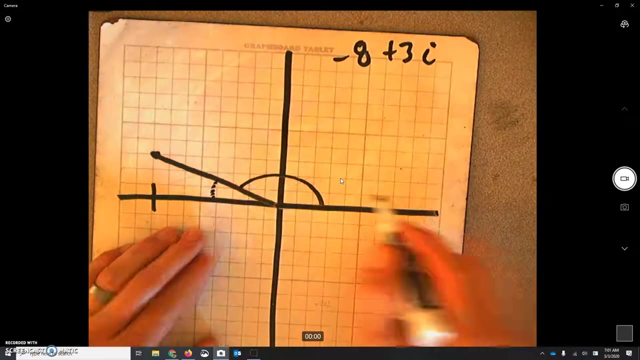 So we want to know what our angle is Right here and it says in radians: Okay. so what we need to do is we need to determine, I want to determine what this angle is And then just subtract this angle from 1 pi. 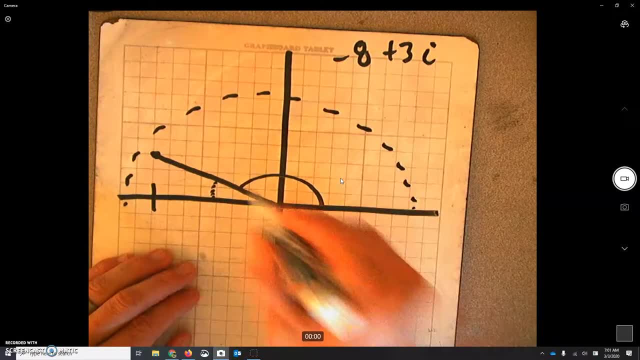 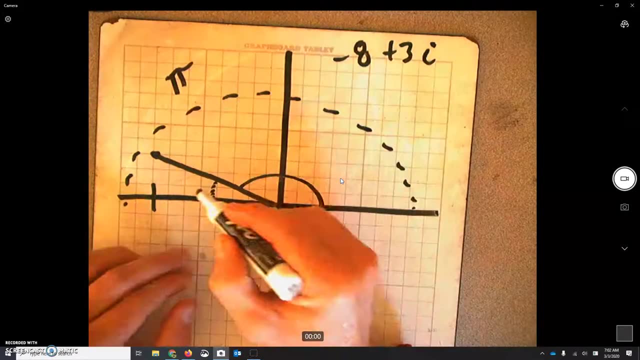 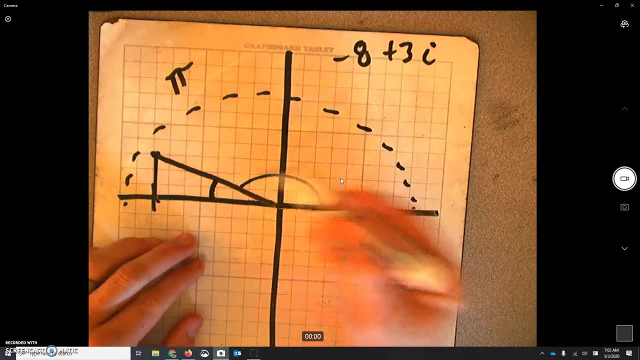 Because, remember, in a unit circle all the way around is just simply 1 pi. So we figure out what this is. We can take pi the entire thing and subtract this chunk and get what we need out of it. Well, how do we find this angle? 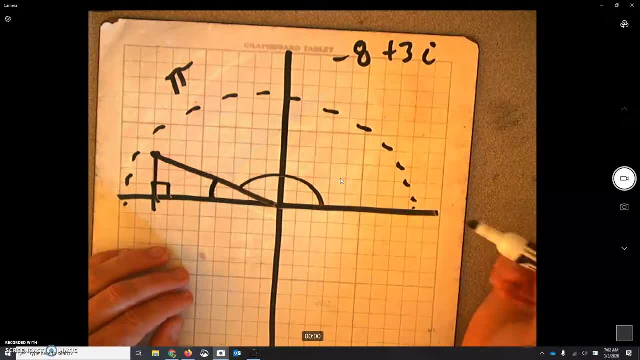 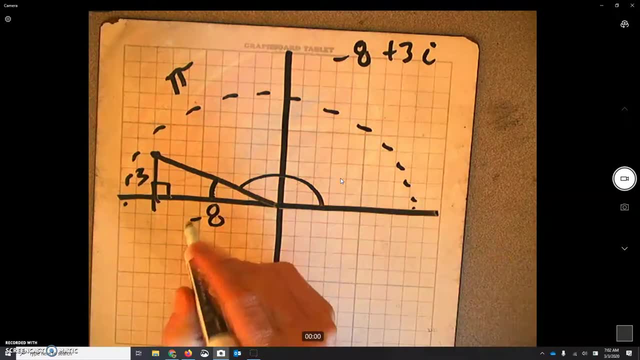 Well, we can use right triangle trigonometry. So this goes up 3, and this goes over negative 8.. We're just going to make it positive 8. Because we're just going to try and find the actual angle of this triangle. 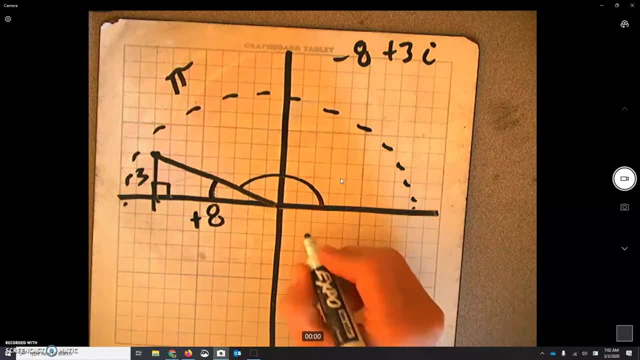 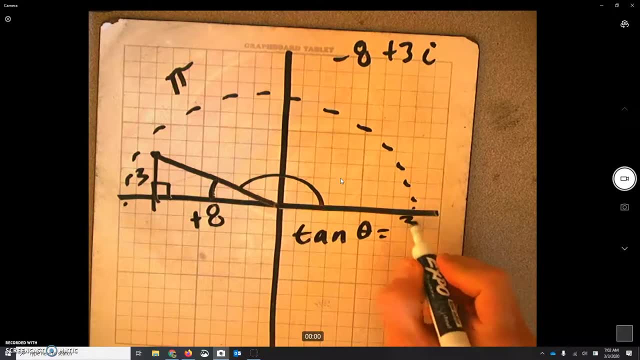 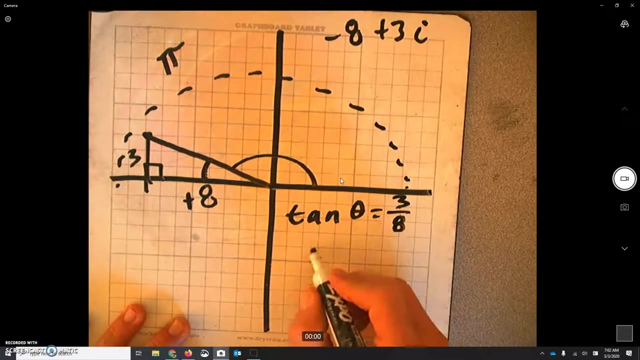 Well, if we don't have a hypotenuse, we can use tangent. So tangent of our angle, theta is equal to opposite over adjacent. And then to solve for theta, we take the inverse tan, So theta is equal to tan of negative 1 and 3 eighths. 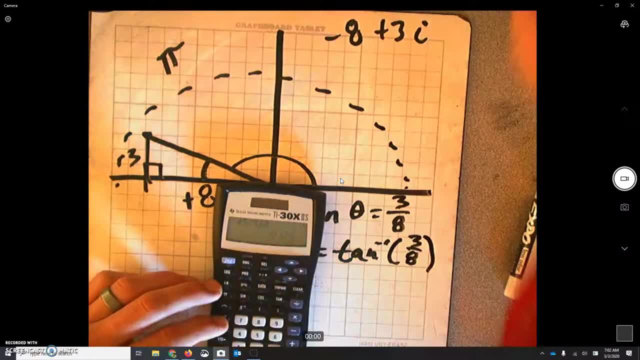 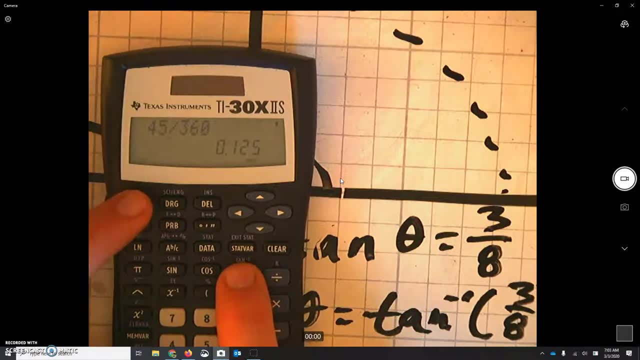 So we do that in our calculator. We have our tan button right here. Zoom in so you can see what I'm doing- And right behind tan we have the inverse tan. So second inverse tan and we're putting in 3 eighths. 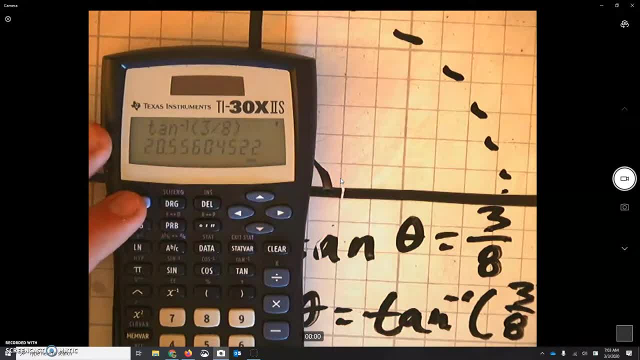 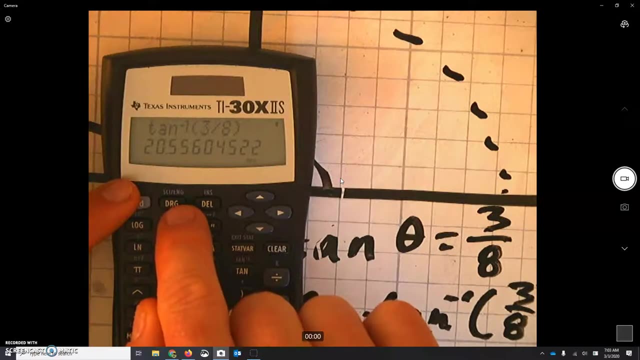 3 divided by 8.. OK, Now this currently is in degrees. I know that because the calculator tells us right here: D-E-G is degrees. If you go right here, it says D-R-G- degrees- radians. and I don't know what the G stands for. 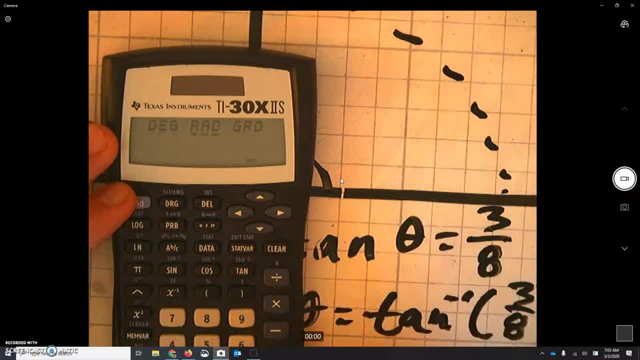 Maybe it's actually just degree up there, I'm not sure. Hit radian and now the same thing and it'll give us in terms of pi, OK, So that's our radian of this angle. Well, we actually want to take, we want our big angle on this side. 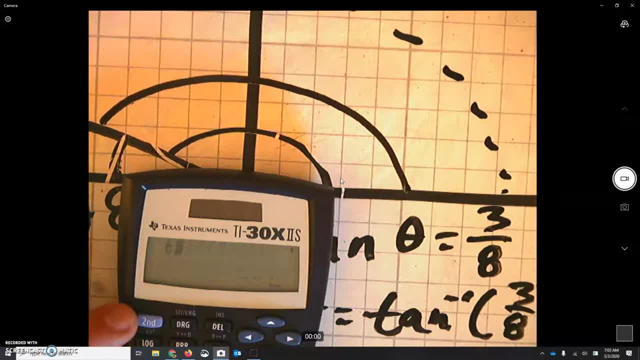 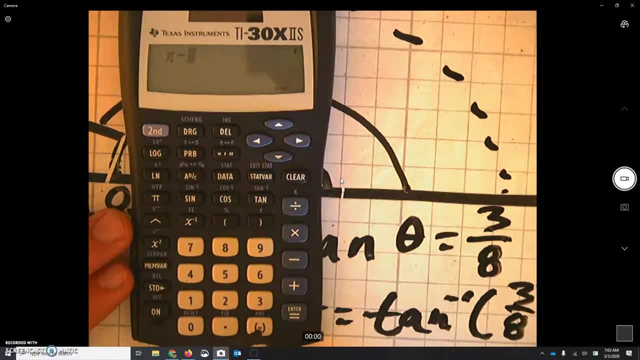 So we're going to do pi minus that. So pi is here, I'm going to subtract and a trick of the calculator down here: A and S. that A and S button copies our previous answer, which is what we had before for our radians. 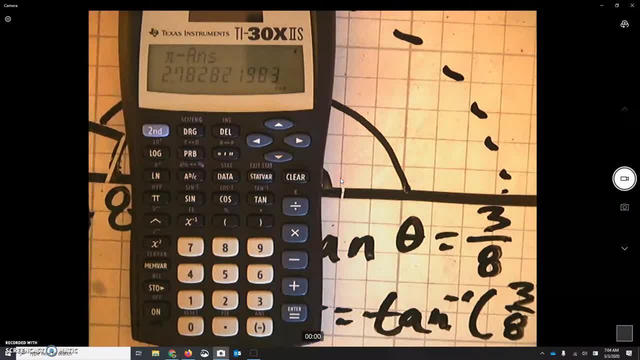 So we'll take second answer and we get 2.7828.. Well, the 2 and the 8, this is 1,000th. This is a 2, so we're looking at the number behind. If it's larger than a 5, we round this 2 up to a 3.. 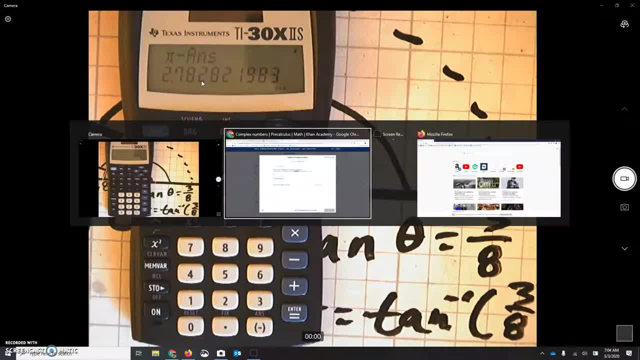 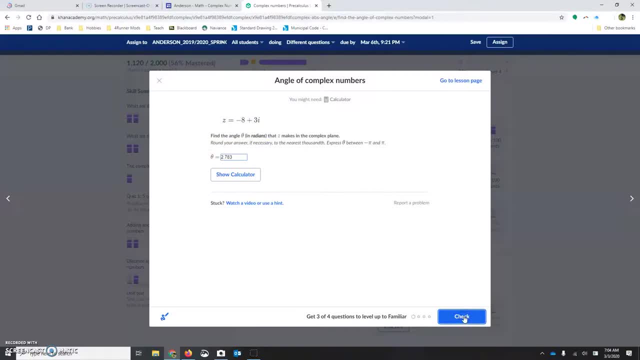 So 2.783.. Remember, 3.14 is a full half circle, so that does make about sense And it's right. OK, I believe the next one will be in degrees. They were going back and forth earlier on these questions.